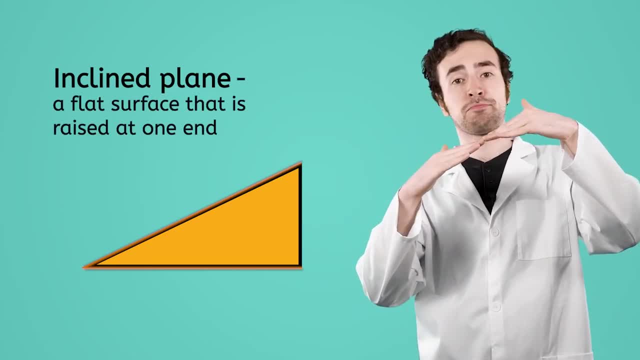 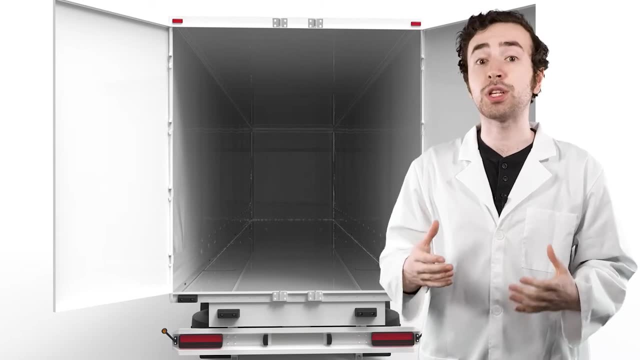 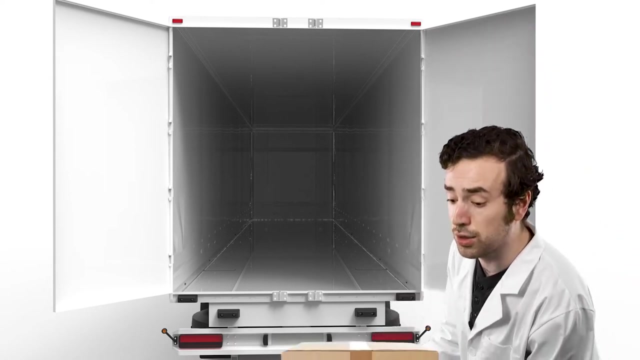 plane is a flat surface that is raised at one end. You might know it by a different name: a ramp. Inclined planes help us move objects between high and low places, For example. if you've ever moved, you might know how difficult it can be to lift a heavy box straight up into the back of a moving. 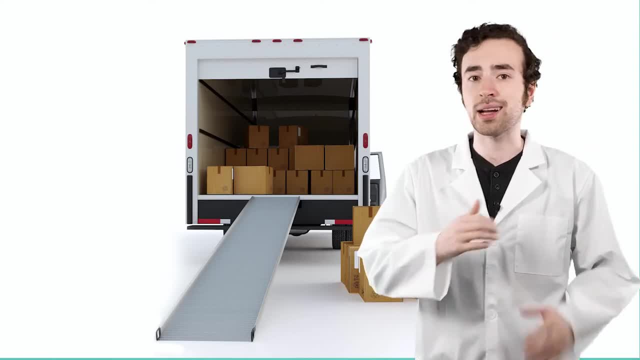 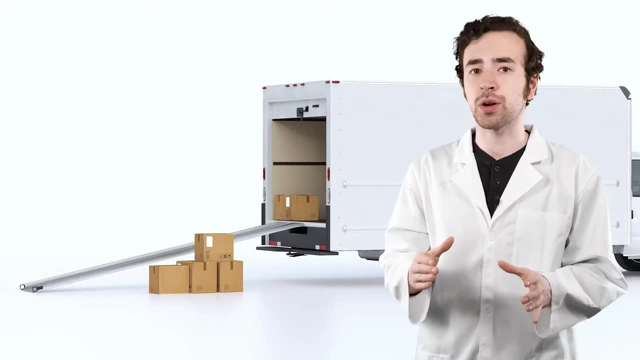 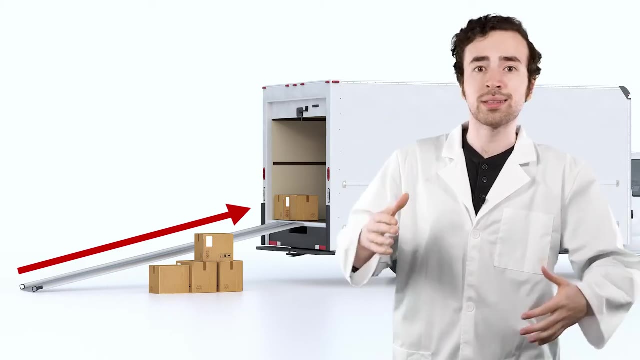 truck. It would be much easier to push that box up an inclined plane into the truck. Inclined planes make work easier by spreading the force we need out over a longer distance. So instead of just picking the box up and lifting it straight into the truck, 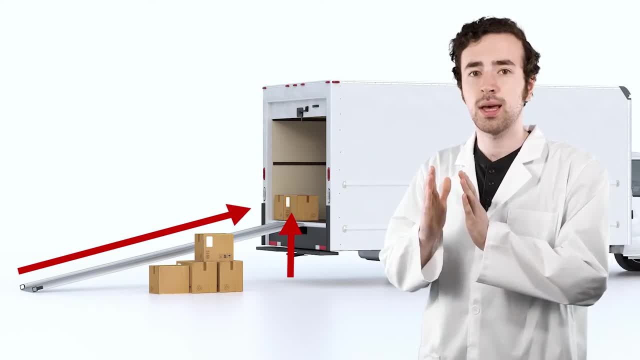 which is a flat surface. you might know how difficult it can be to lift a heavy box straight into the back of a moving truck. It would be much easier to push that box up. an inclined plane into a large amount of effort. over a very short distance The inclined plane spreads that. 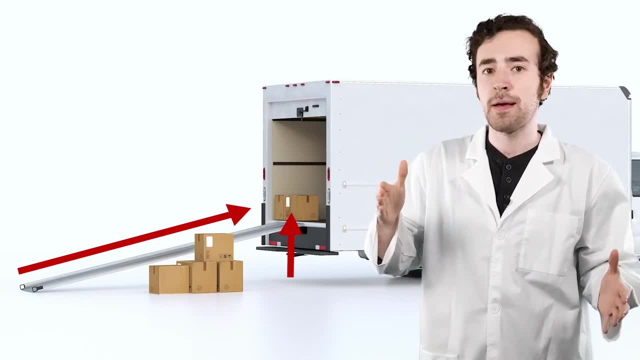 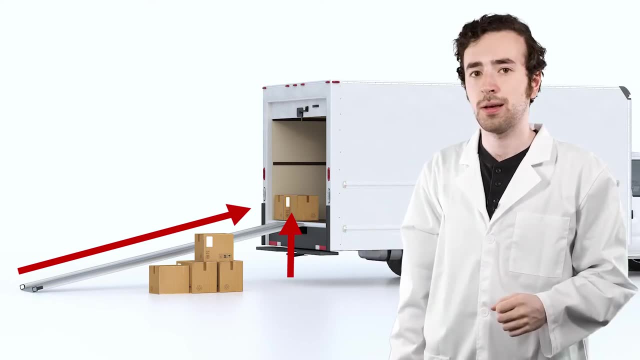 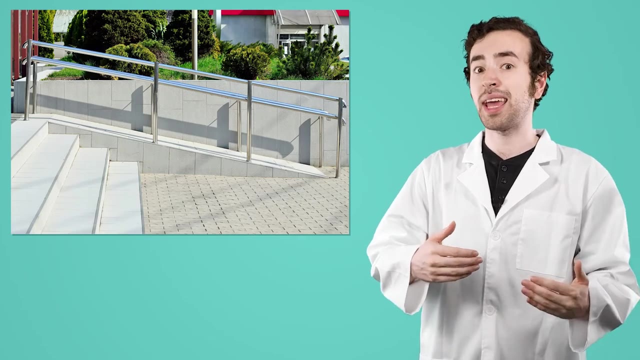 effort out over the length of the ramp, meaning that we can exert less force as we gradually push that box into the truck. This is probably why it feels easier to go up an accessibility ramp rather than a steep flight of stairs, or why hiking trails usually wrap around the 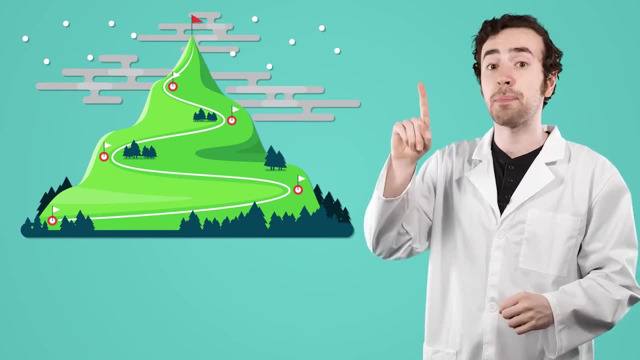 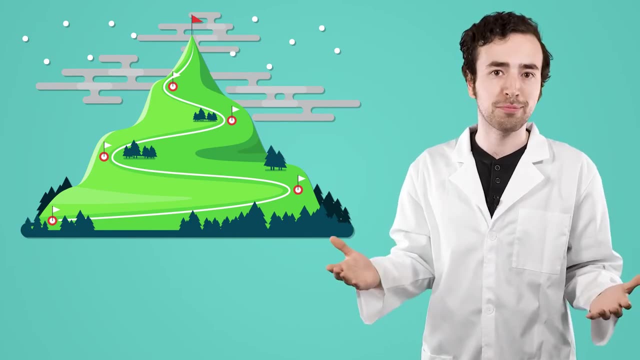 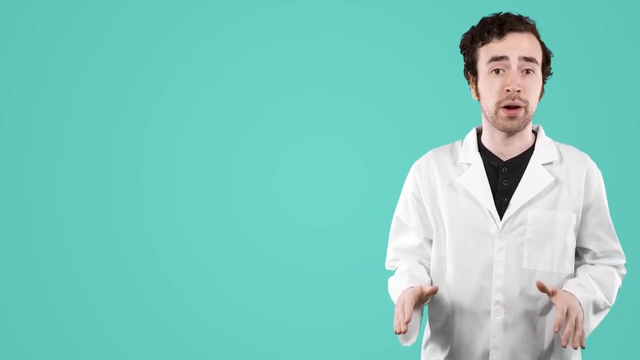 side of a mountain instead of just going straight up it. By extending the distance, the force we need to do the work is spread out As one of the simplest of the simple. machines. inclined planes are everywhere: Curb ramps on sidewalks, book shoots at your local library. 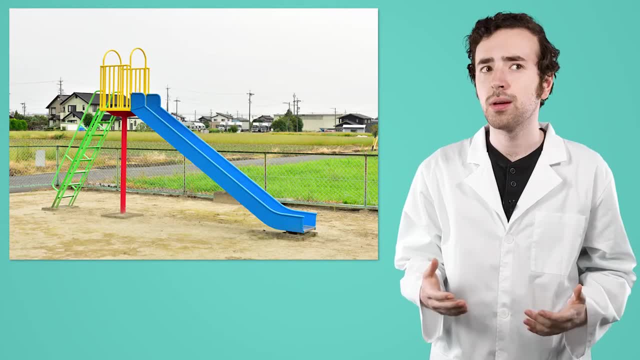 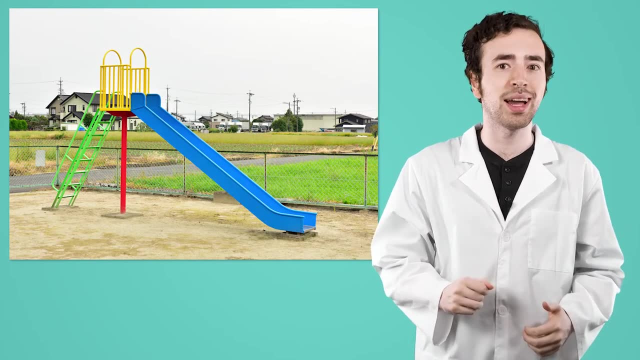 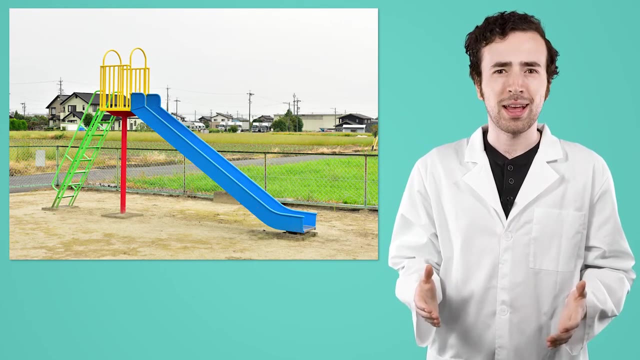 even slides on a playground. Actually, that's a great way to put an inclined plane in my treehouse. I'll put in a slide so it's much easier to get to the ground than climbing down the ladder. Fantastic. Where are other examples of inclined planes that you've seen? Pause the. 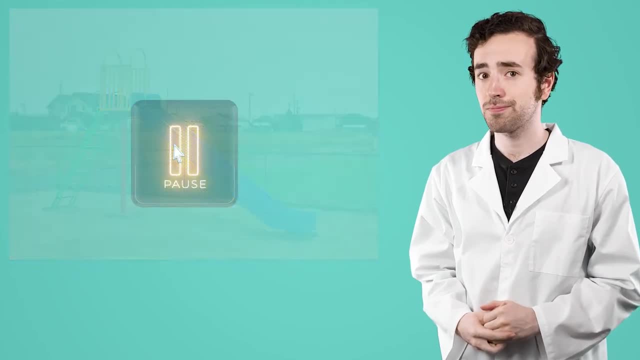 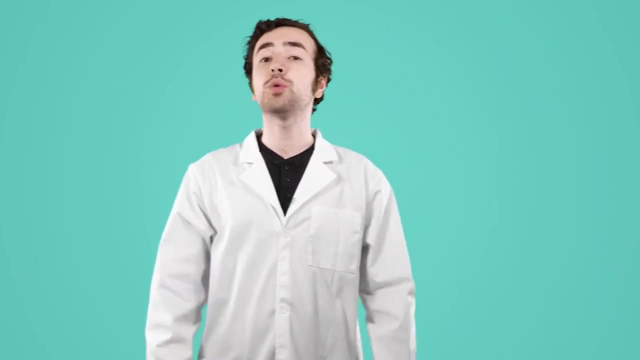 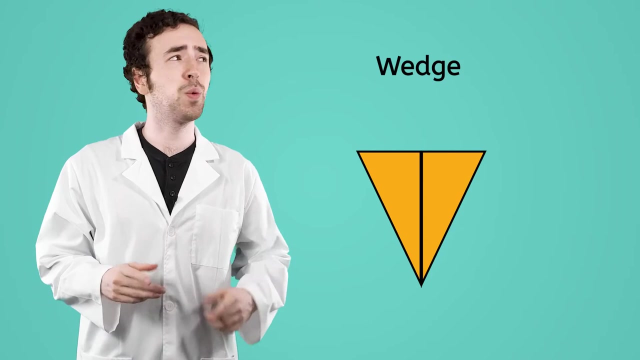 video here to jot down your thoughts in your guided notes. So now that we've got the inclined plane down, it's time to move on to our next simple machine, the wedge. No, you're not seeing things. The wedge is very similar to an inclined plane. It's kind of just. 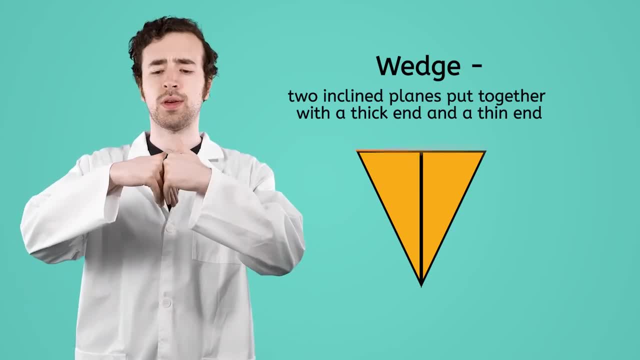 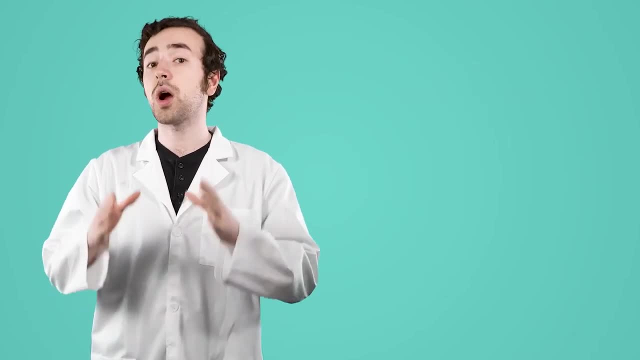 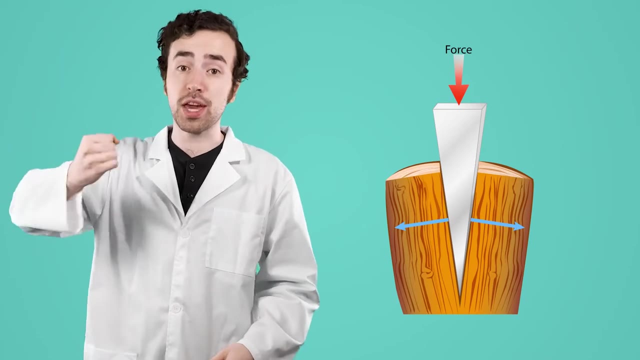 two inclined planes glued together with a thick end and a thin end. The difference is how they're used. Wedges are used to break objects apart, like wood. Force is applied to the thick end of the wedge, which pushes the thin end into the thin end of the wedge. 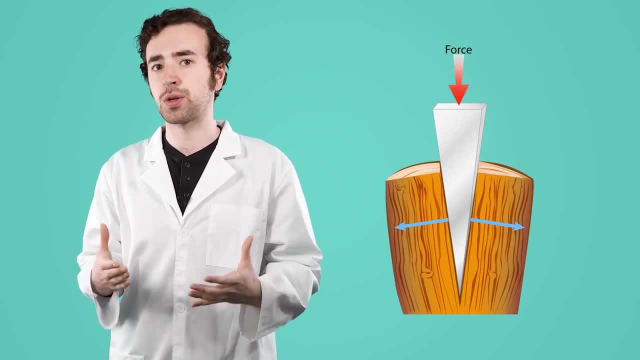 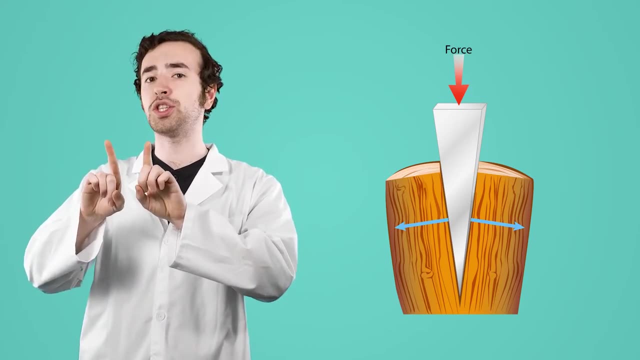 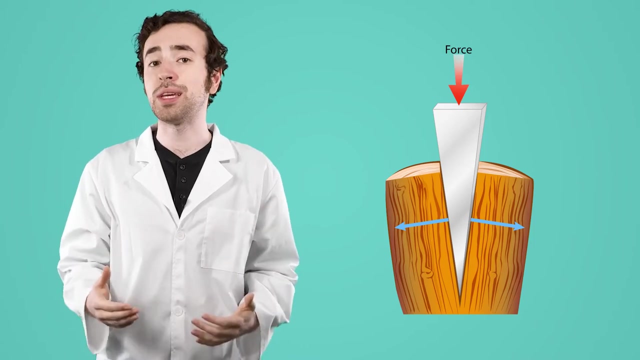 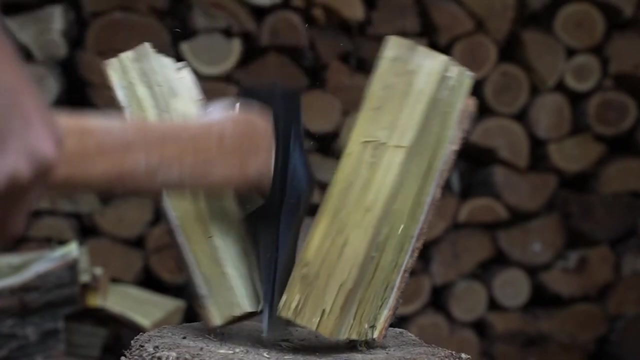 The wedge redirects the force applied, sending it outward. This in turn pushes the wood up against the wedge's inclined planes, breaking it apart. Wedges make breaking things into smaller pieces much easier. An axe used for chopping wood is a classic example of a wedge, but wood is. 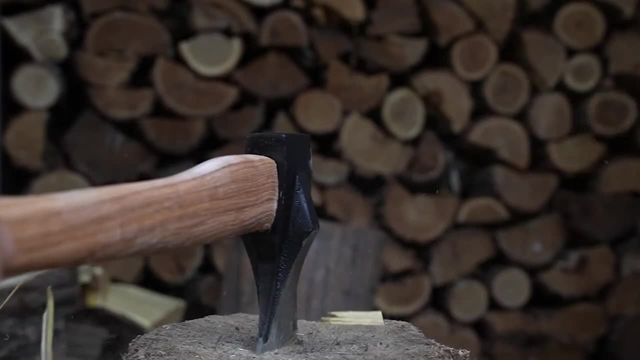 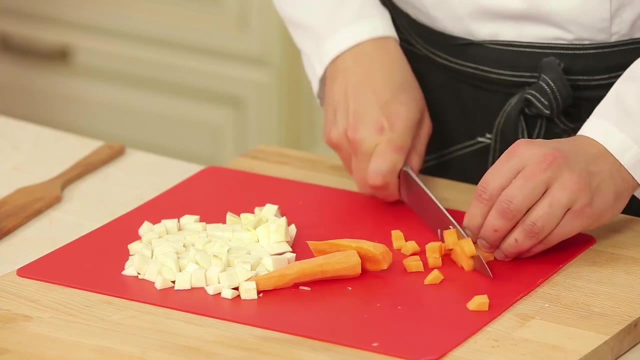 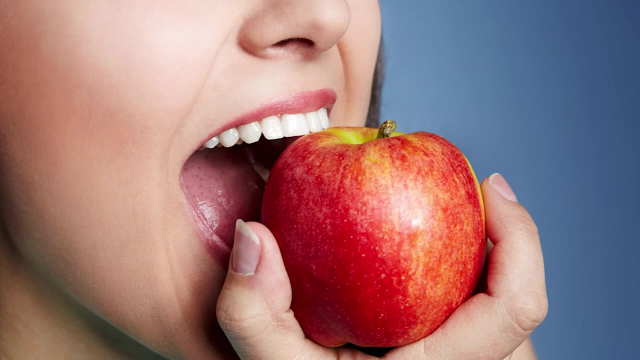 certainly not the only material that can be used to chop wood. The wedge is used to chop wood into smaller pieces. A kitchen knife, for example, is a very thin wedge, and it cuts food apart in the same way. an axe cuts wood. Your front teeth actually work the same way. Pay attention to how. 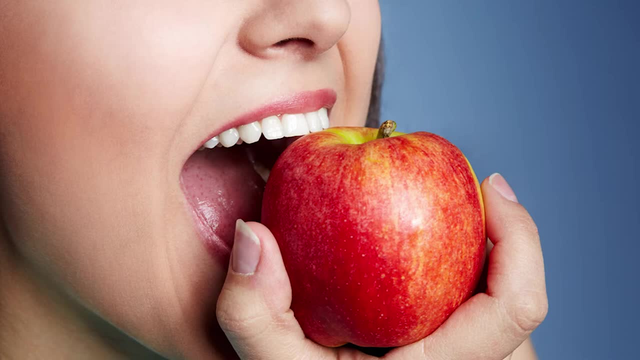 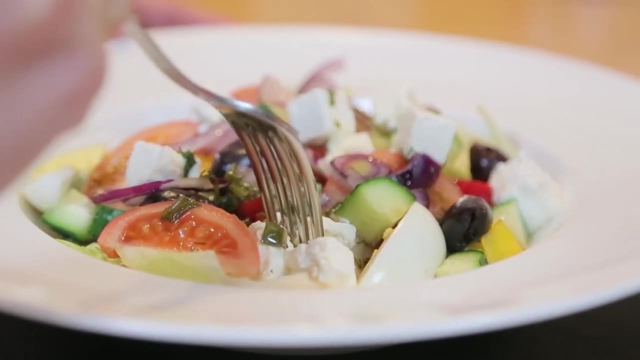 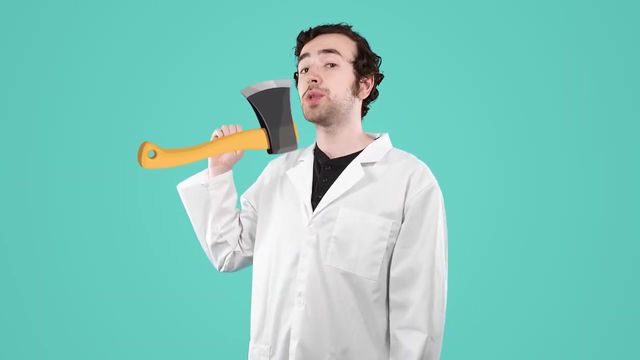 they split food apart the next time you bite into an apple. Even the tines of a fork, when you look very closely, are wedges, making it easier to pierce food than it would be without them. As for me, I think I'm going to be using a wedge in the construction of my treehouse by using an axe. 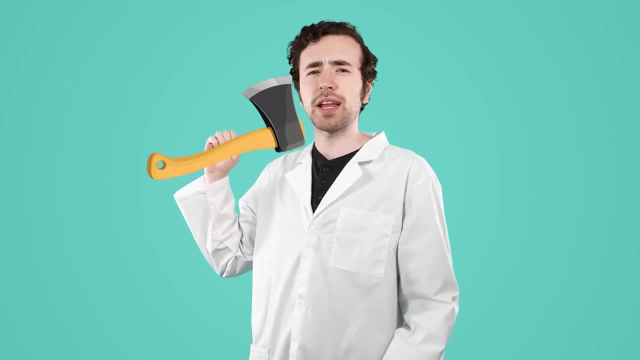 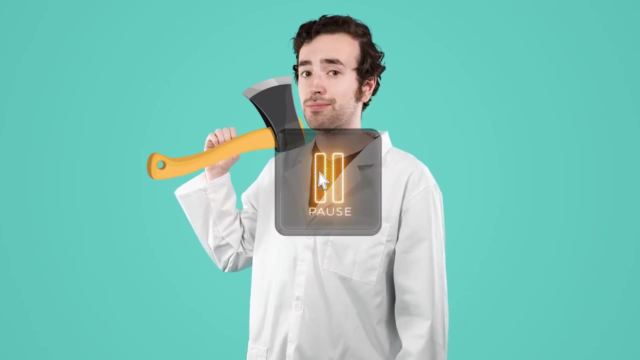 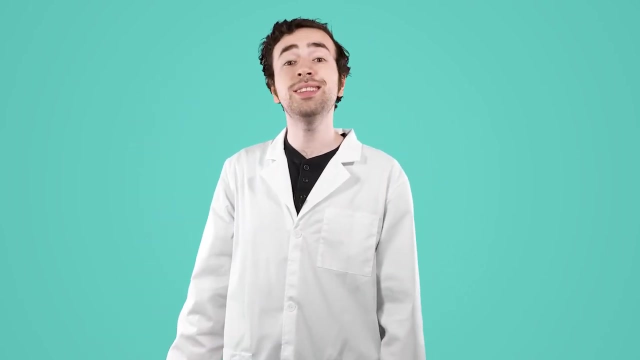 to chop the wood I need for it. Can you think of any other wedges I might want in my treehouse? Pause the video here to jot down your answers in your guided notes. Now, our final simple machine for today is the screw. Now, if you look closely, 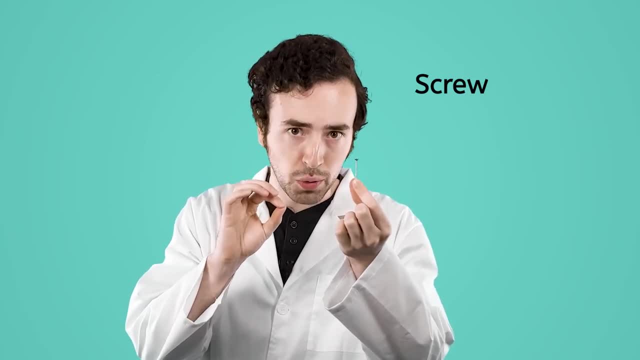 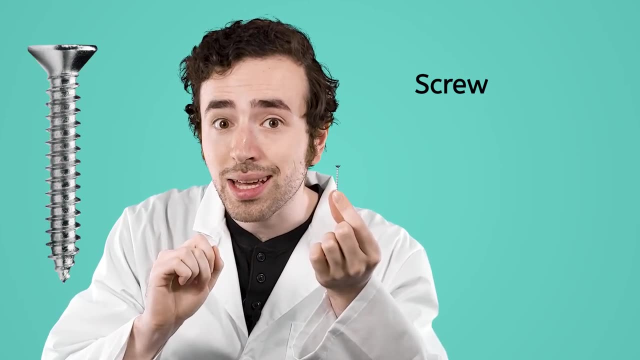 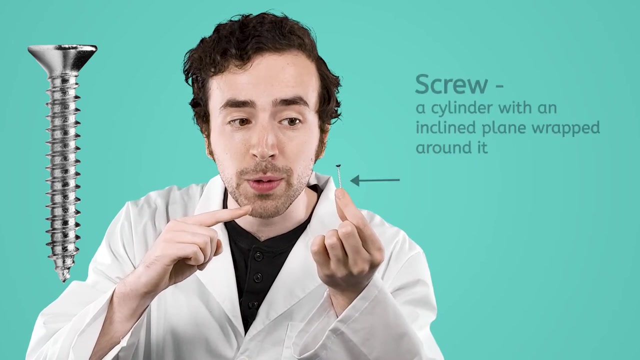 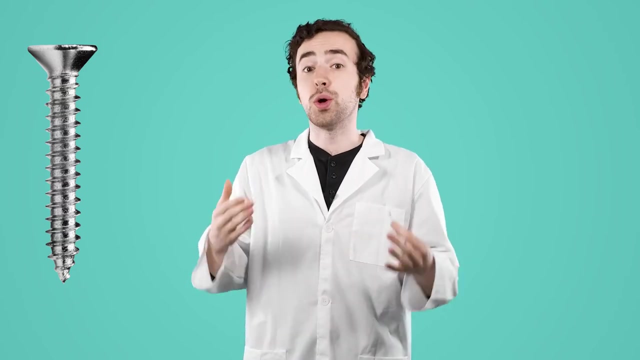 you can actually see that a screw uses an inclined plane. A screw is just a cylinder with an inclined plane wrapped around it in a spiral. Screws can help us with all sorts of things. They can hold objects together, drill holes or even lift heavy objects. 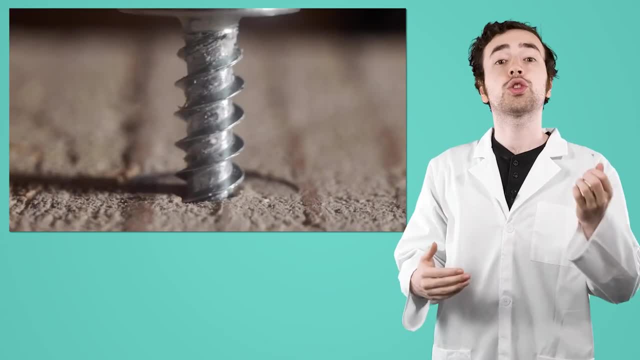 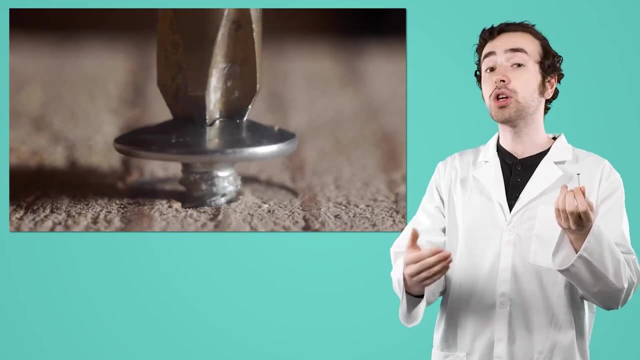 Just like inclined planes, you can also use a screw to chop wood. So if you look at the planes and wedges, screws help make work easier by changing the direction of the force applied to them, which pushes objects up. that inclined plane spiraled around it. 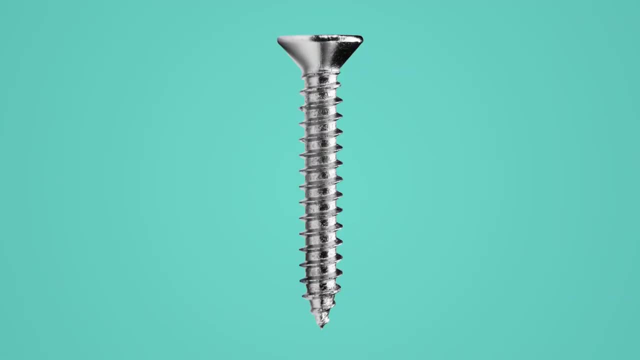 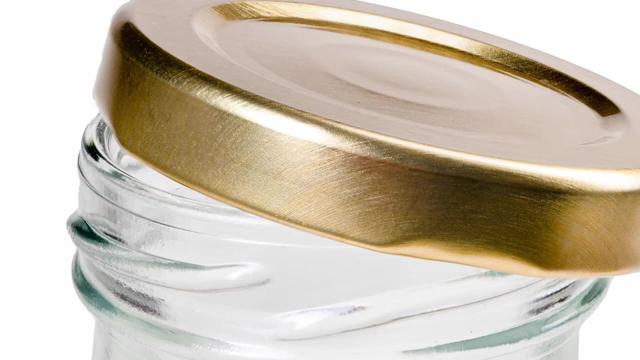 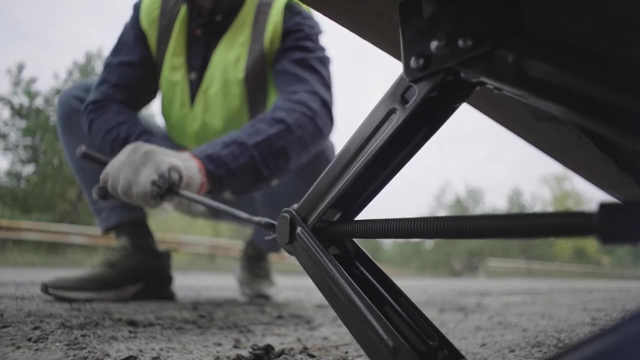 You can find screws used to hold things together almost anywhere you look. Light bulbs, bottle caps and jar lids- all use this simple machine to securely hold their pieces together. Machines like jackscrews use a screw to lift extremely heavy loads. Scientists even use 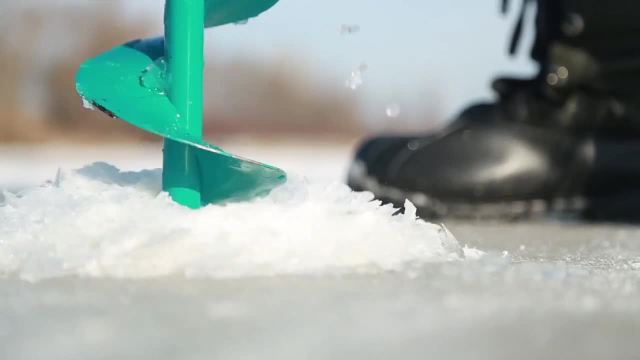 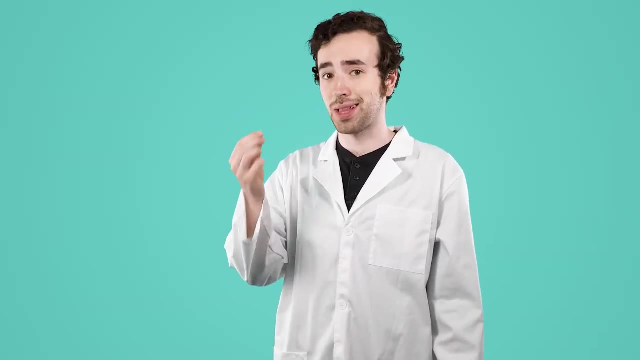 screws to pull samples of ice to study from deep within glaciers. Despite all the amazing ways we use screws, I think I'm just going to stick with the classic. for this one, I'm going to use metal screws to hold all the pieces of wood together that I need. 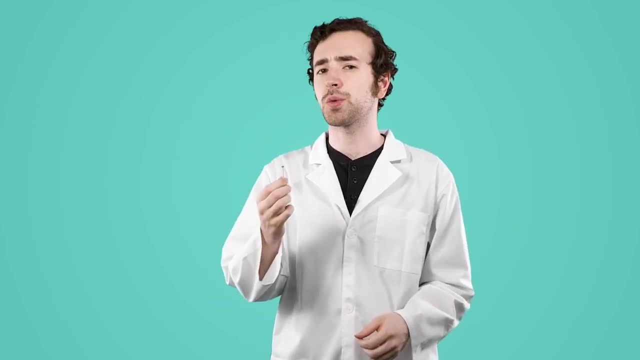 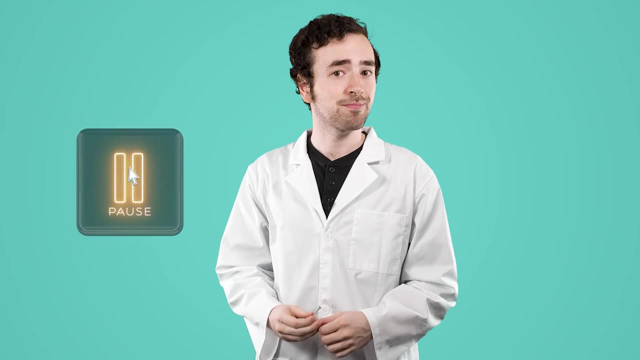 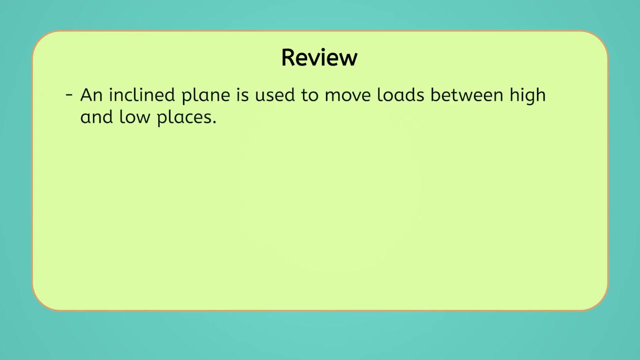 for my treehouse. Can you think of any other places we use screws? Pause the video here to write down your ideas in your guided notes. Let's review everything we've learned today about the last three simple machines. An inclined plane or ramp is used to move loads between high and low places. 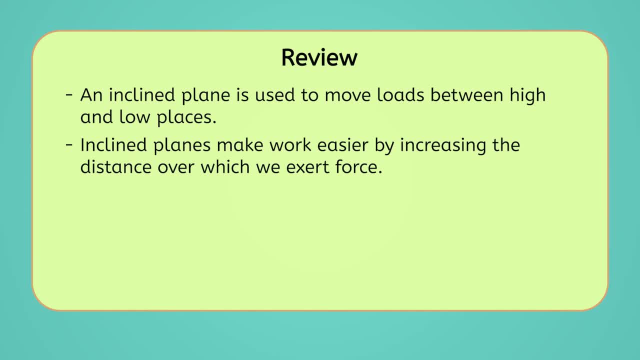 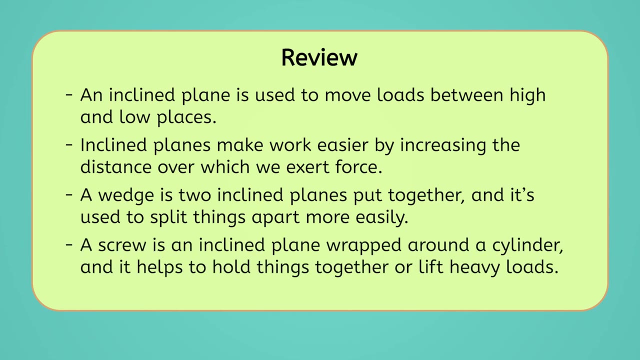 It makes work easier by increasing the distance we exert force over. A wedge is two inclined planes put together and it's used to split things apart more easily. A screw is an inclined plane wrapped around a cylinder and it helps to hold things together or lift heavy loads. 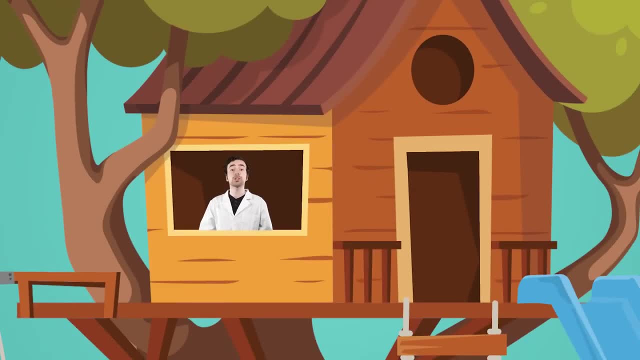 To learn more about inclined planes, wedges and screws, be sure to check out the activities and practice questions for this lesson. As for me, thanks to the power of simple machines, I now have an amazing new treehouse to study in. I'll see you again soon. 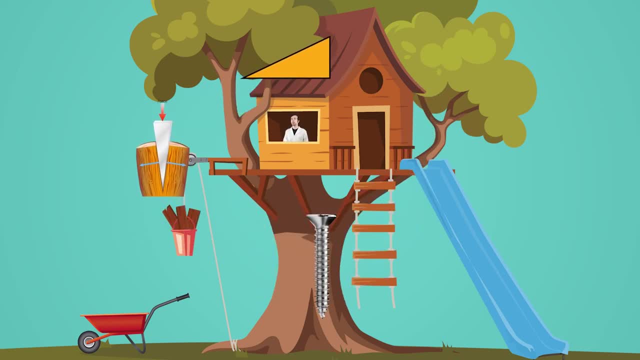 but until then, And remember, science is all around us. See you next time.